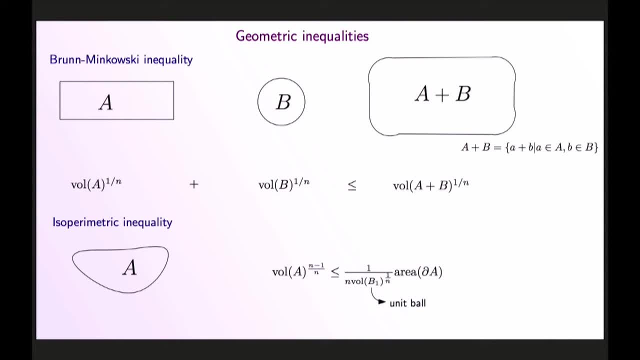 And the second is a parametric inequality. So the Brunnen-Kovsky inequality relates the volume of two sets with the volume of the sum of two sets and the sum is just point-wise sum, the Minkowski sum of two sets. 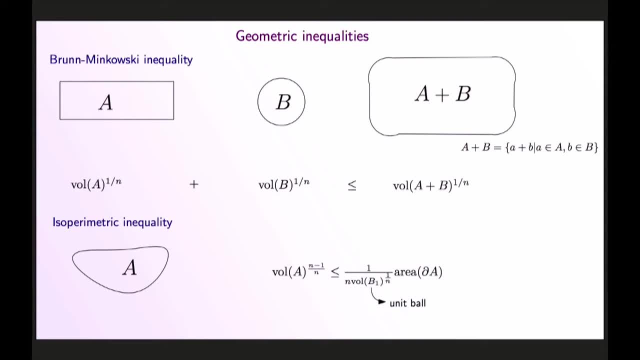 The either parametric inequality relates the volume of the set and the area of the boundary. So this is the boundary, With some normalization given by a unit boundary. So how can we relate this to classical information theory? So in geometry we have sets. 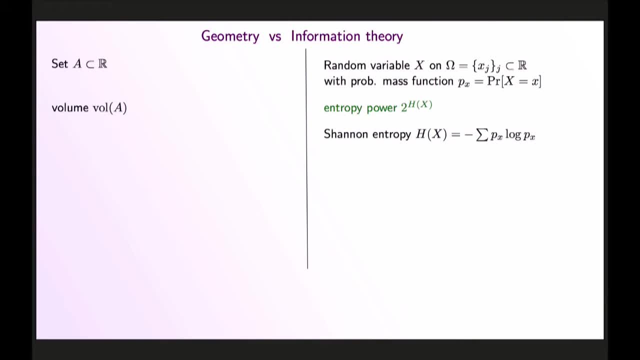 And in classical information theory we have random variables, So one is going to be associated with another. For the volume, we're going to be associated with an entropy power. And why is that So? here the entropy power is power of the entropy. 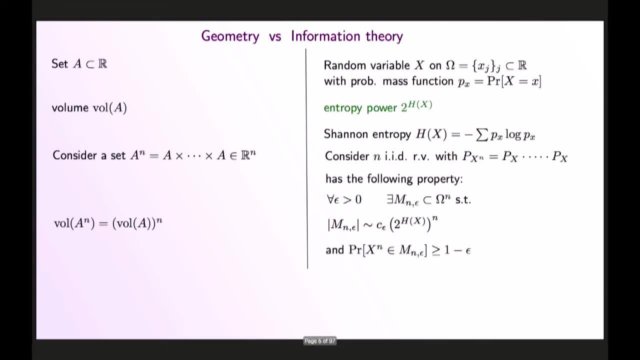 This is a Shannon entropy. So why do we associate entropy power with volume? Because the scaling is similar. So if you consider a set in Rn, just a multiplication of a given set, the volume is going to be the power. 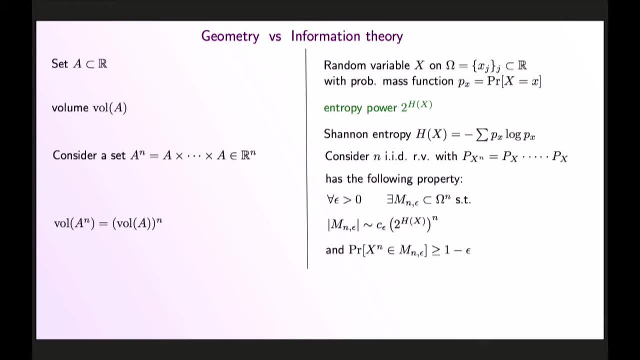 Now if you look at the IID random variables, it has the following property: that it mostly concentrated on a set that scales as power of the entropy power. So your new IID random variables, Xn, is mostly concentrated in the set that scales as the power of the entropy power. 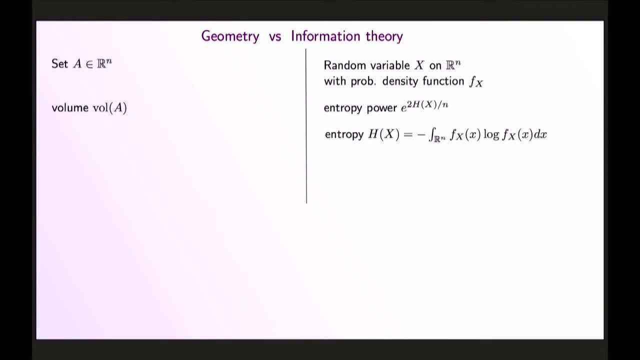 So on Rn we have a random variable, And here I'm going to have a log, natural log. so a natural power instead of two. It's a variance of a Gaussian random variable with the same entropy. So this is just a notation, just a different notation. 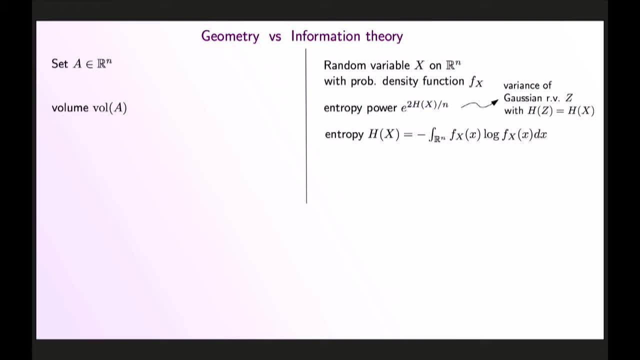 So this is n dimensions now. That's why we have a scaling of n And the entropy is this integral. Now, in the previous slide we had a sum of two sets. We also have a sum of two density functions, a sum of two random variables. 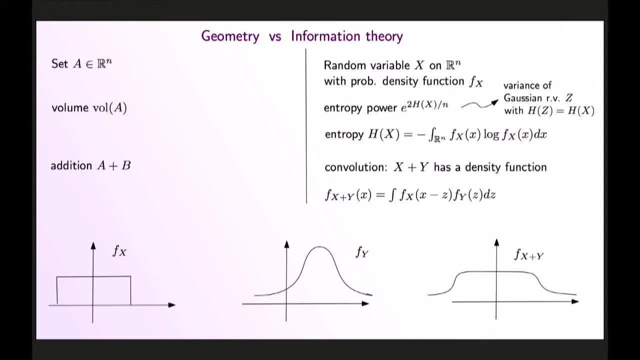 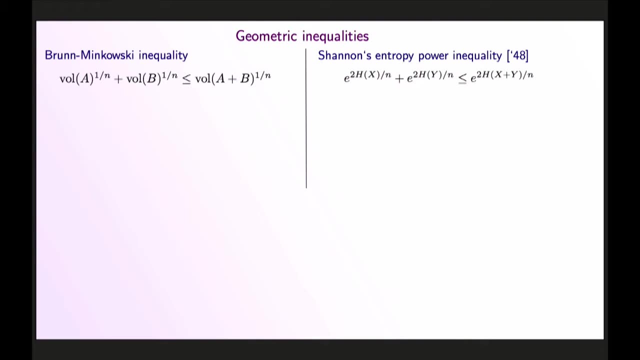 And the density function is given as a convolution. So that's a picture for the convolution. So okay, now we have everything set, We can generalize the inequality to the classical information inequality. So the Brin-Minkowski inequality related the sum of two sets with the volume of the sum. 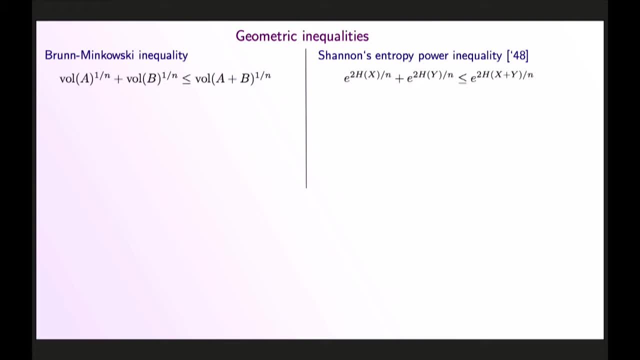 And in the classical information we relate the entropy powers, which were just like volumes, with the volume of the sum of two random variables, And the result was proposed by Shannon. and then several works will prove that The second inequality is isoparametric inequality. 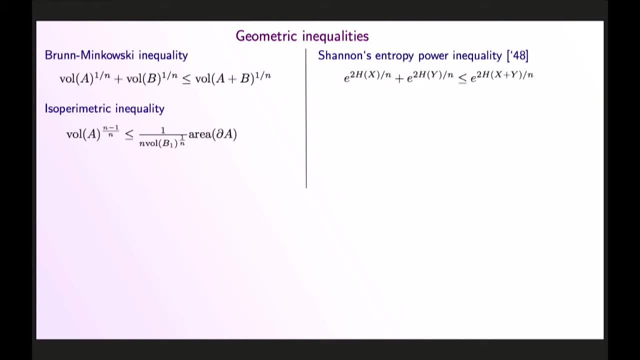 It's like this one, But the problem here is with area of the boundary. What is its analog to classical information theory? So the volumes we have, for the volumes is the entropy power, But what's the area of the boundary? So let's look at the proof of the isoparametric inequality and see what happens there. 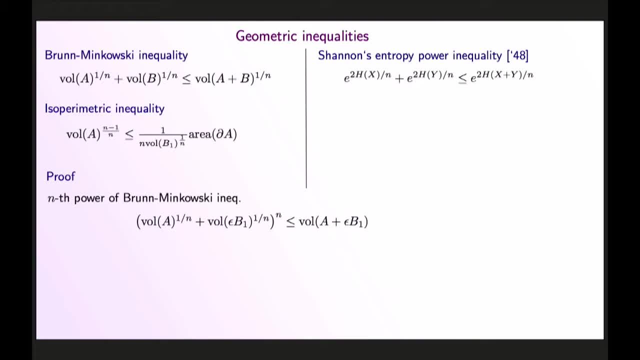 So the proof relies on the Brin-Minkowski inequality. Let's take this inequality to power n, And instead of set B we're going to have an epsilon of a ball. B1 is a ball, It's a unit ball. 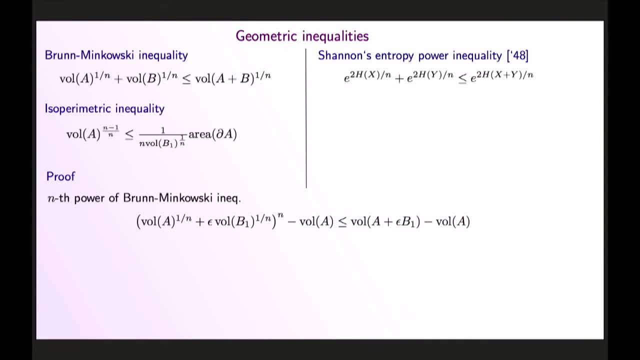 Okay, so that's the nth power. If I subtract the volume of A, well, that's all I did, just subtracted volume of A and took a limit- epsilon- going to zero. Okay, so what happens On the right-hand side? this is exactly the area of the boundary. 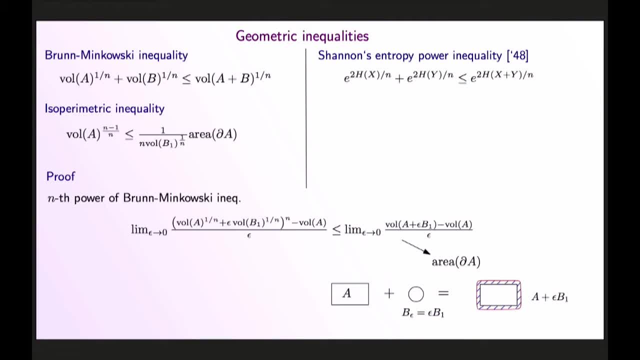 We have a set. We added an epsilon of a unit ball, just a little bit expanded our set, We took the limit and we get the area of the boundary. But now what happens here on the left-hand side? So you see, this is just a derivative of the volume. 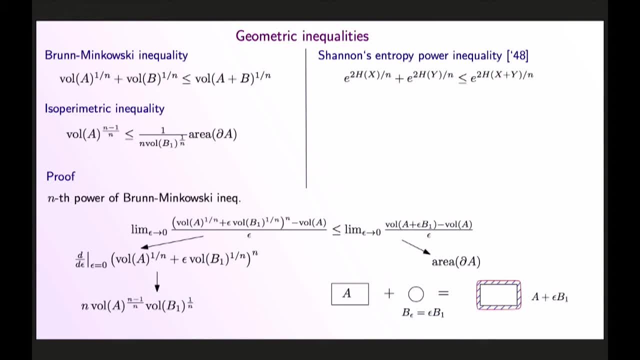 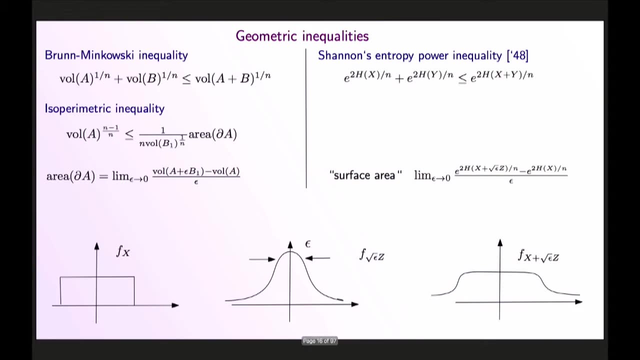 So this is the derivative of this whole stuff, Because when epsilon is zero, you just have a volume of A. So if you take the derivative and calculate it, this is what you have. Okay, so now we can do the same thing in classical information. 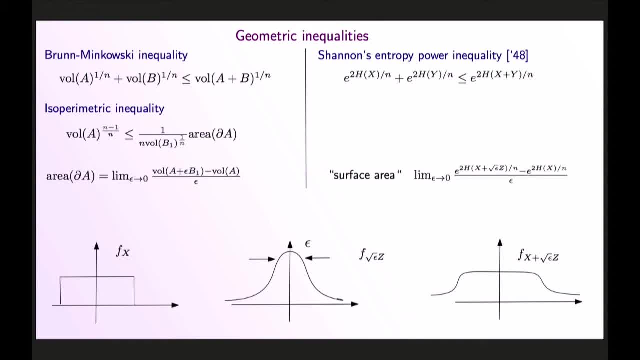 So the area, we have this limit for the area, So the same thing we can call a surface area, is a limit of the difference of entropy powers when X is summed with the Gaussian random variable, So Z is a Gaussian random variable and I multiply it by square root of epsilon. 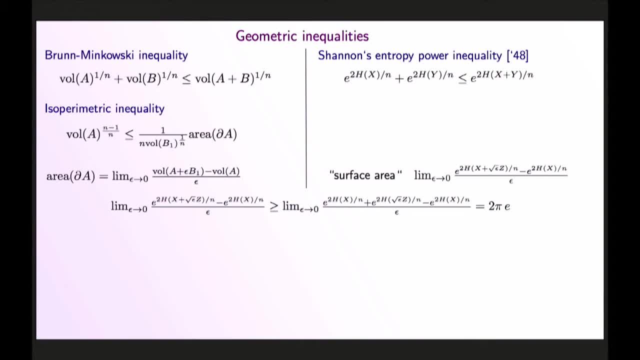 So that's my new surface area. Okay, so what can I say about it? So, the first term, I can use the Shannon entropy power and bound it from below by the sum. So you see, then, the first and the last term came. 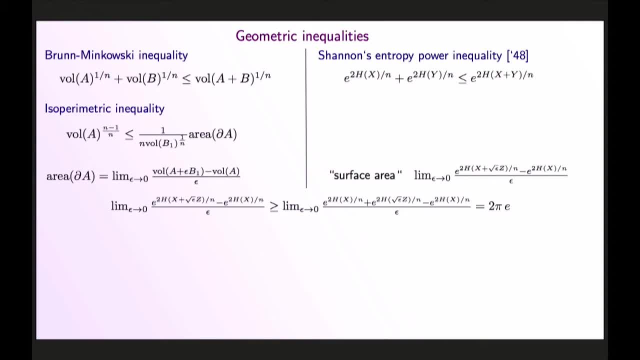 So the first term cancels. I can take epsilon going to infinity, calculate it and get 2 pi E, But on the left-hand side. so what's going on on the left-hand side? On the left-hand side, this is a derivative of the entropy power. 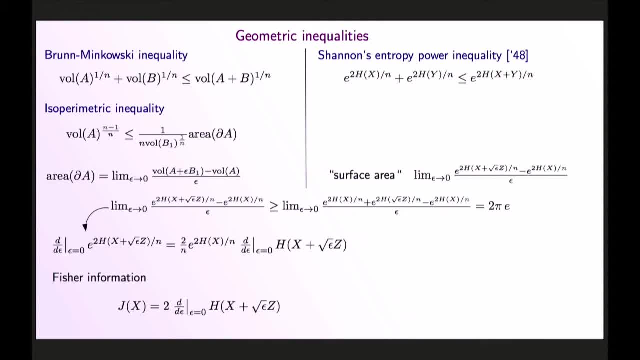 Okay, let's take the derivative. So you take the derivative, You're going to have the derivative of the entropy. Now let's just denote this derivative of entropy as something called J of X, a Fisher information. Okay, So then my inequality, isoparametric inequality. 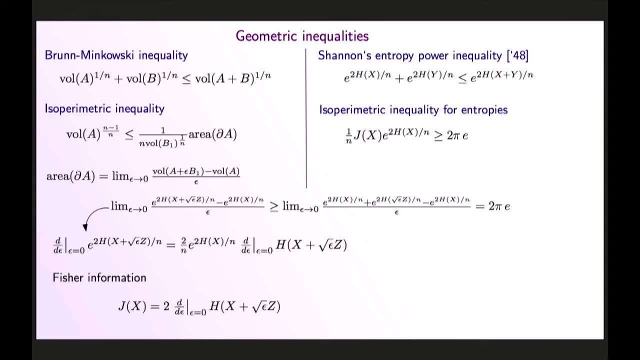 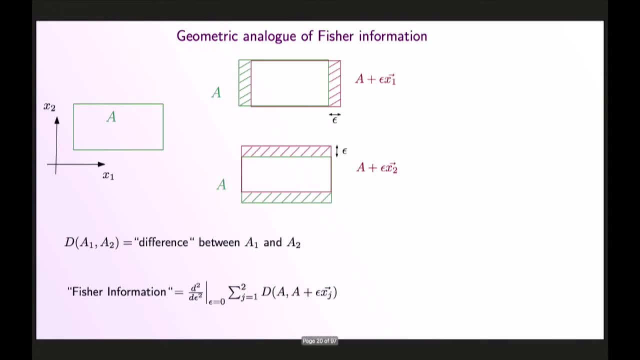 is going to look like this, And that's what's called isoparametric inequalities for entropies. But now let's focus on the Fisher information. So I call that Fisher information And in geometric sense this is the following: 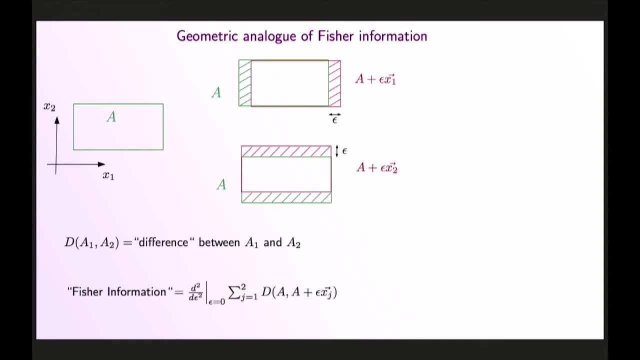 So you take a set A. Well, let's take in two dimensions here And we translate it a little bit in each dimension, Just by a little bit. Then if I have some notion of a difference between two sets, then the Fisher information is going to be the second derivative. 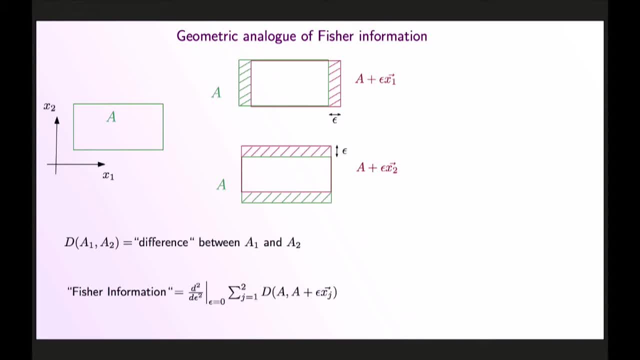 of all possible differences between my set and the new translated one. Oops, sorry. So for the classic confirmation theory, the Fisher information is going to be a second derivative of a distance between my function, my probability distribution, with some sort of a translated function. 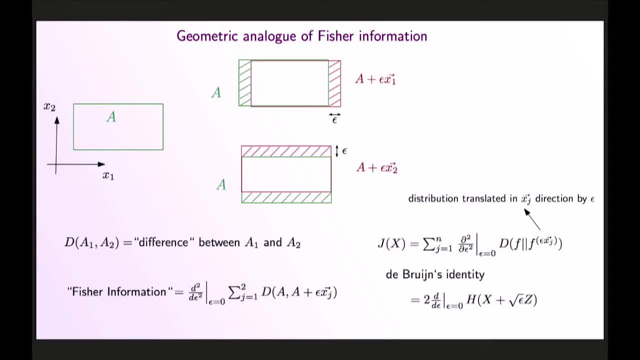 And I will talk about it later, right? So this is just an idea of what it is, And it turns out to be equal to a derivative of the entropy, And this is called de Bruijn's identity, This relation. It's a separate one. 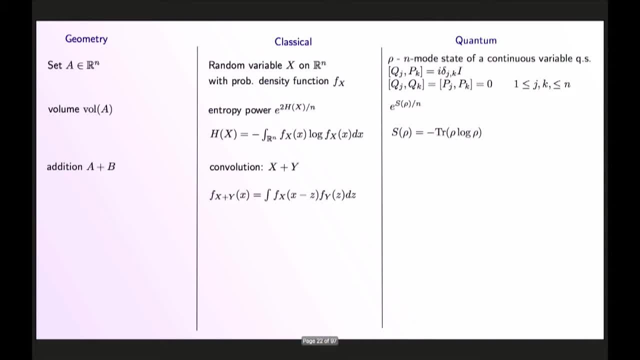 Okay, So that was a classic confirmation theory. How can we translate that to quantum information theory? Okay, So in quantum information theory we had sets which correspond to random variables in classical information theory. In quantum theory they correspond to states, obviously. 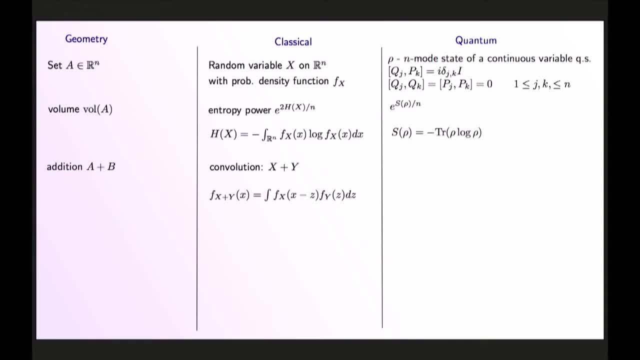 And let's take n-mode states here, And we're going to take them bisonic states with q and p satisfy the canonical commutation relations. Now for the volume. we had entropy power in classical. Well, let's take an entropy power in quantum. 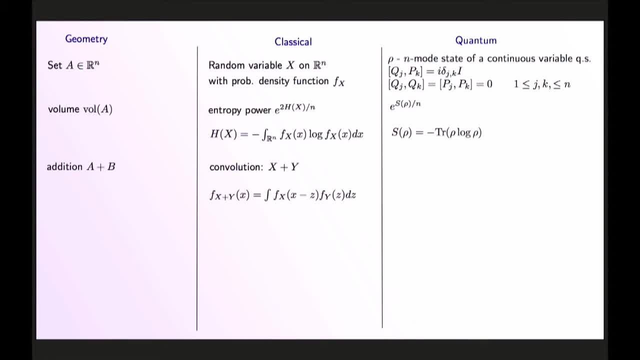 Two. So my entropy here is binomial entropy. Now you see there is a little bit difference here with coefficient two. This is just due to dimensions here, Because n-mode state correspond to two n-mode state in classical one. That's why you have a difference of two. 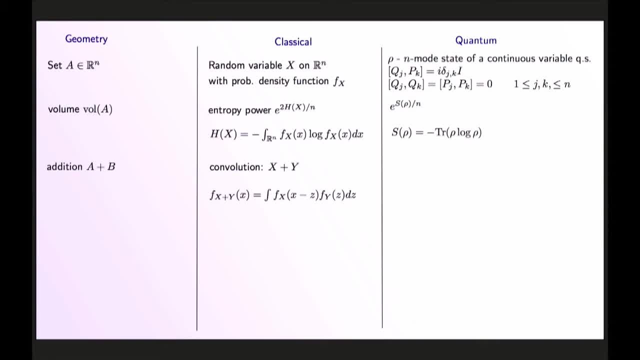 That's fine. Okay, Now for addition of two sets. we had a sum of two random variables which corresponded to a convolution between two probability distributions. Now how can we add two quantum states? So what would correspond to adding two quantum states? 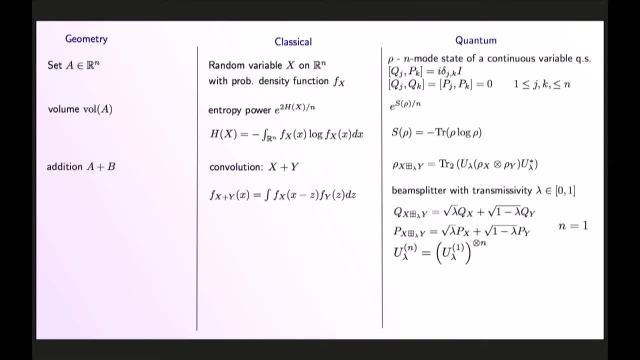 So one of the proposals is to use a beam splitter. So the beam splitter, we saw it in the previous talks this morning. So this is the definition of a beam splitter. You send two states, x and y, and you ended up with one mixed up together. 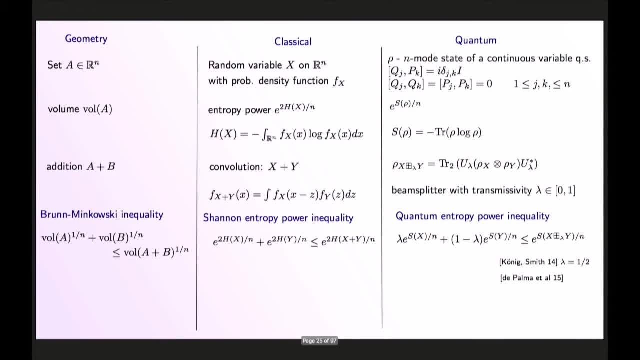 Okay, So for this beam splitter, the analog of the entropy power, inequality was proved in 2014 and 15 in the following way: So we had the Brummenkowski inequality relating volumes. Here we have entropy power relating the sum. 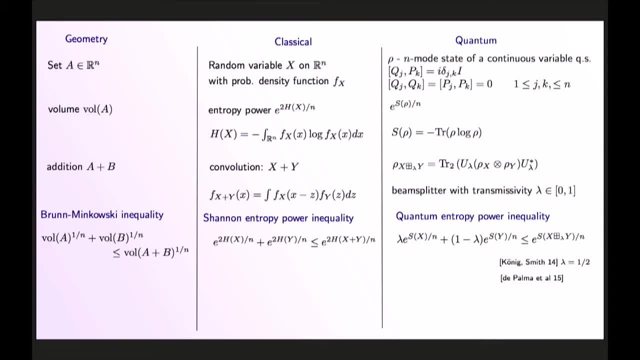 of two random variables. And here we have the entropy power relating the end result of a beam splitter operation with two original states. And the coefficient lambda correspond to coefficient of the beam splitter. But now for the second inequality, the isoparametric inequality. 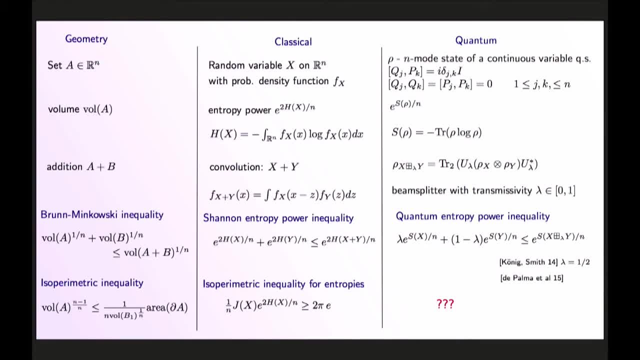 the analog is not so obvious. You cannot just generalize the classical setting into quantum one. So the proposal is, our proposal is the following- is to do something in between, to take a classical state and the quantum one. So we call it classical quantum convolution. 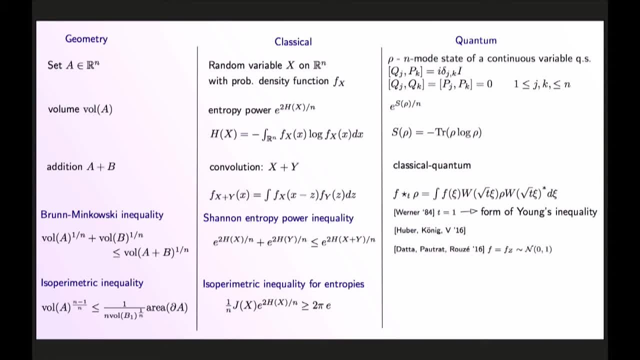 It was introduced by Werner in 84. And he derived a form of Young's inequality. And then in our two papers that I'm reporting on, we considered it general with coefficient t. In the second one it took a Gaussian, a random variable. 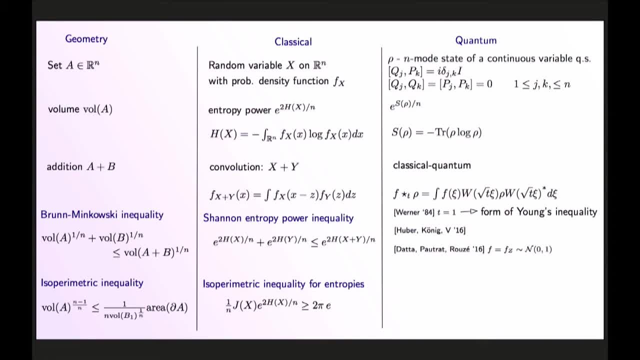 So for that quantum classical convolution we can derive both entropy power inequality and the isoparametric inequality. So here we have the classical input, quantum one, and the result, And here it's true for all quantum states. 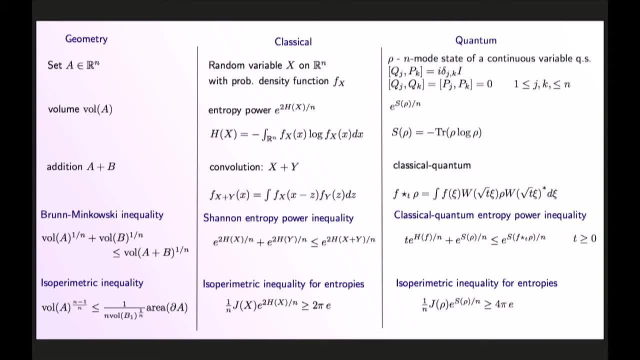 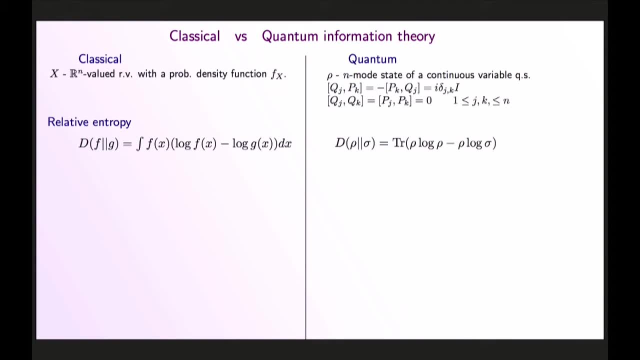 So it does not depend on the convolution at all. Okay, so let's start a bit more precisely on the information theory. So again, we had a classical random variables And the quantum states. So we saw before we had a relative entropy. 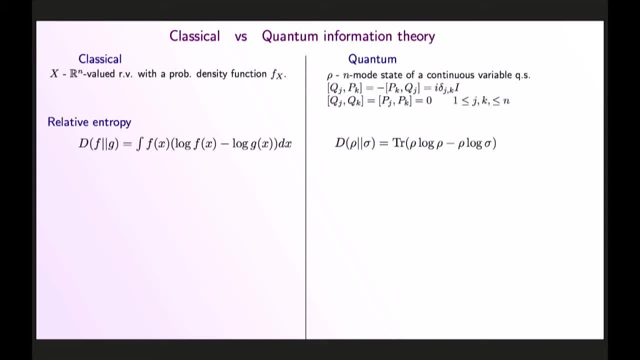 So this is a relative entropy for the classical and the quantum one. So the Fisher information in classical defined as follows: So you translate your function f, just by taking, just by translating it in x axis, Now taking a relative entropy as: 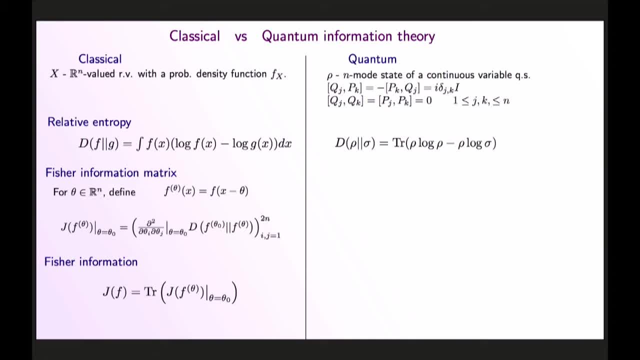 the measure of difference between your two functions. you take a second derivatives of all the translations and you take a trace That is going to be your Fisher information. Now you can translate that to quantum setting. but then the question is, what is the translation of my function or my state? 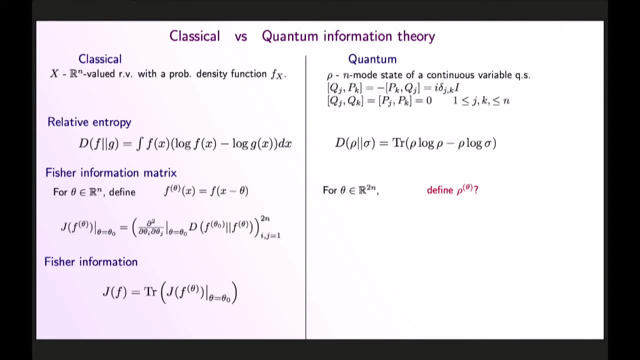 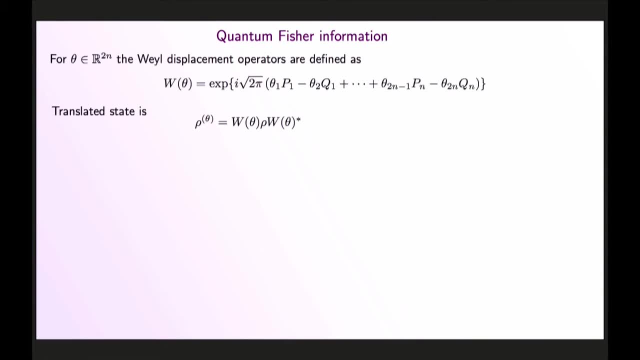 So how can we define the translation? Well, one of the way to do it is to use Weyl's displacement operators, And the Weyl's displacement operator is defined in the following way: So we have a vector theta, which is this theta: 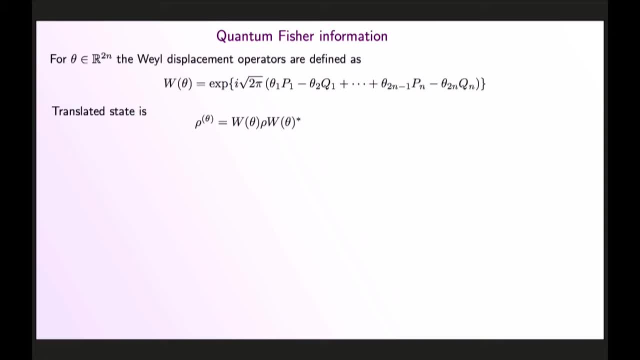 So, and by each of these coefficient, p is taken with plus signs and q is taken with minus signs. The translated state is then going to be just that one. You translate it with Weyl operators. sandwich it there. The property of Weyl operators is that. 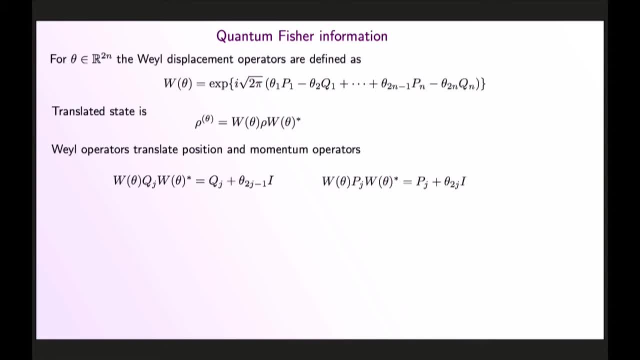 why they translate. they translate q and p's, So they're a good choice for translation, because you just translate it by identity for q and p. So the Fisher information matrix is just like before. It's defined as second derivatives of the relative entropy. 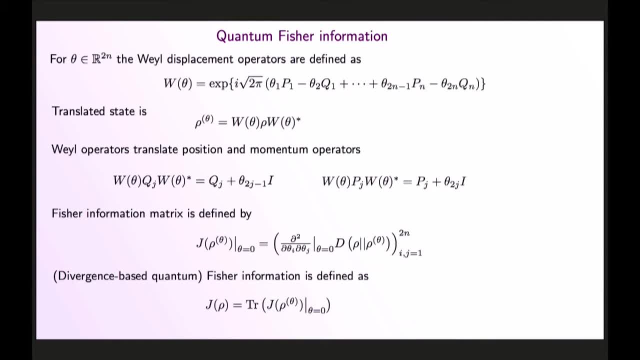 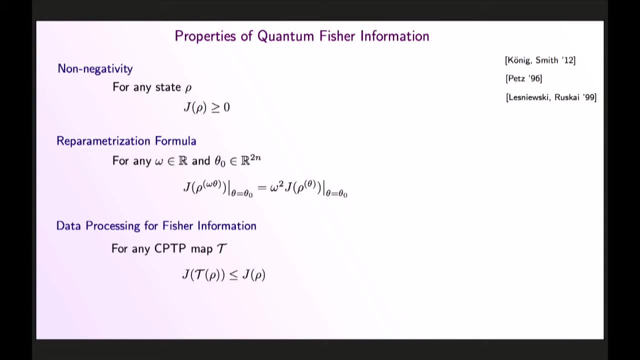 and the Fisher information as a trace. Now, what are the properties of the Fisher information? And first I need to tell you that it was studied previously by Petz in 86 and Ruskay and Lisnevsky in 99 as a Riemannian metric. 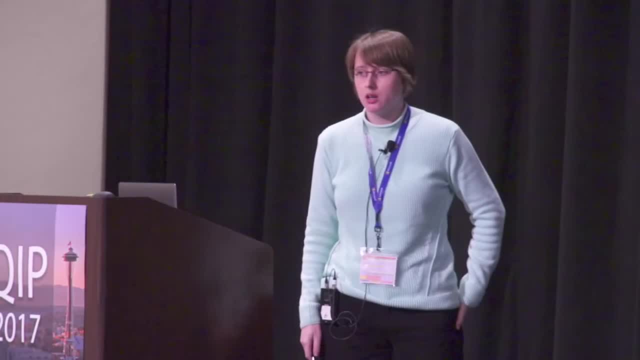 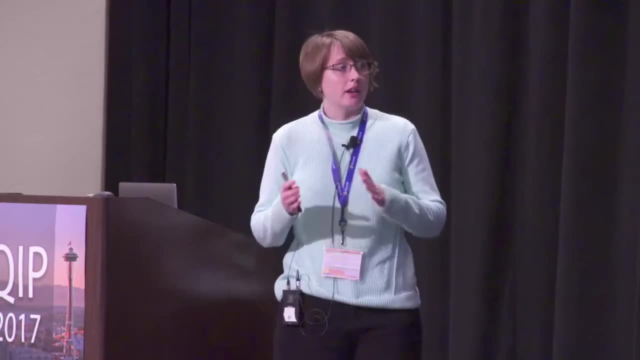 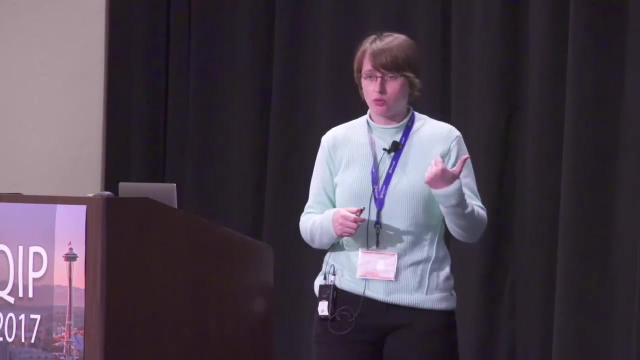 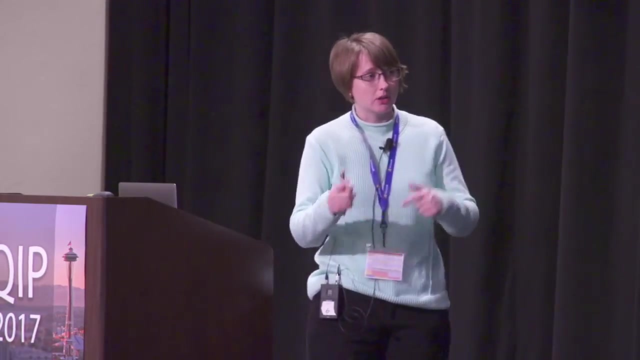 And they showed a one-to-one correspondence between monotone metrics and monotone operator functions. They also showed that all Riemannian metrics are derived in this way, in a similar way to the way we derived divergence-based Fisher information, And that Fisher information is monotone. 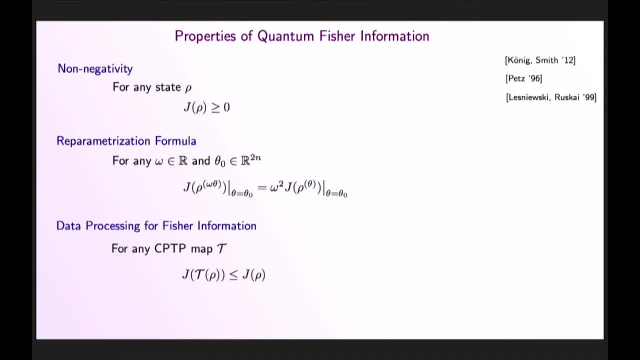 Also Koenig-Smith independently proved all these properties directly for this particular divergence-based Fisher information. So it's non-negative. You can pull out this coefficient omega and it's monotone where it satisfies the data processing inequality. So for any completely positive, 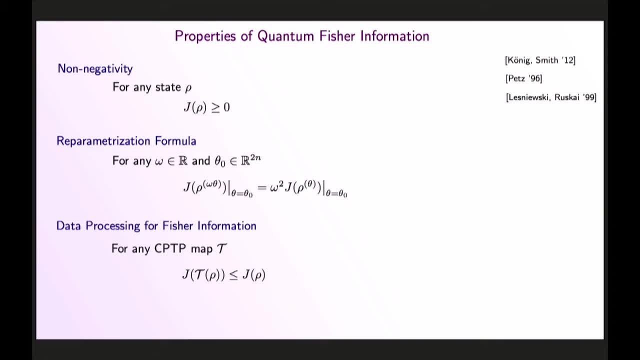 3x7 map. you're going to do worse on the output. Okay, so for the convolution itself. so again, it was introduced by Werner, for t equals 1, and then we generalize it for any t For such a convolution. 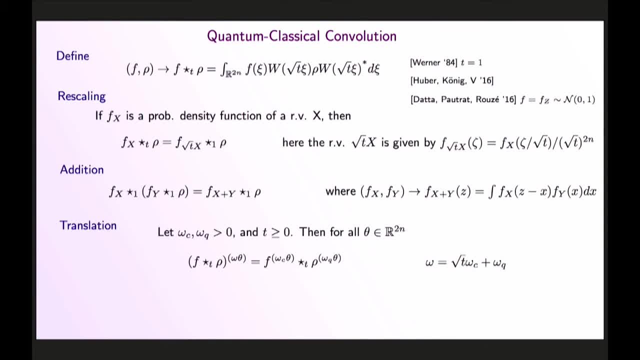 the simple properties are the following: So you can rescale this t, So you can move this t to x and take the convolution with 1, when t equals 1.. And here the rescaling is the usual rescaling of the random variable. 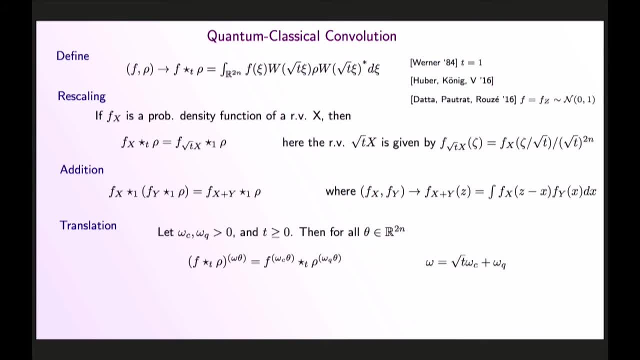 Now you can add, You can make two convolutions in a row. It's going to be just adding of two random variables And you can also translate. So if I use a translation which was defined using while operators, it means that we first translate our function. 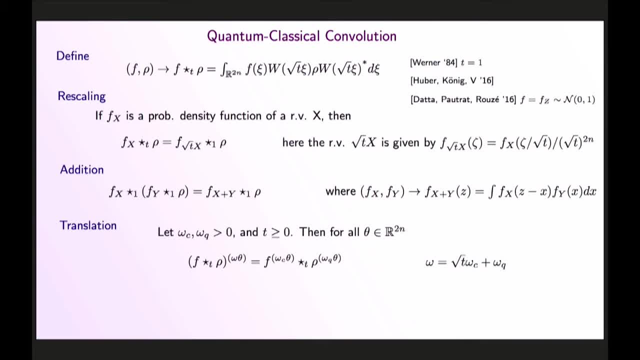 our probability density function and then we translate the state. So it's the same one And there's a relation between all three coefficients. And then there is an important property which we rely on in all our proofs: It's a data processing inequality. 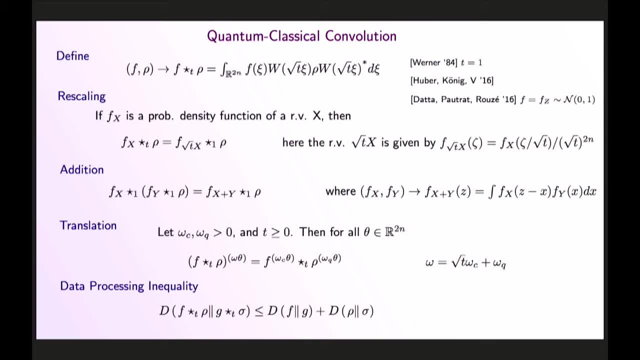 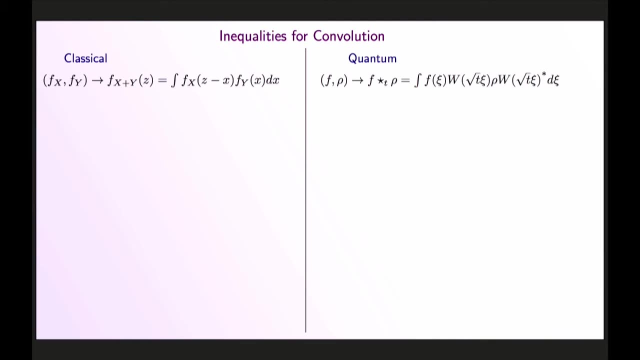 It shows that the relative entropy between two convoluted states is less than the relative entropy between two classical functions and two quantum states. Okay, So what are the inequalities for both convolutions? So in classical we use just a regular convolution. 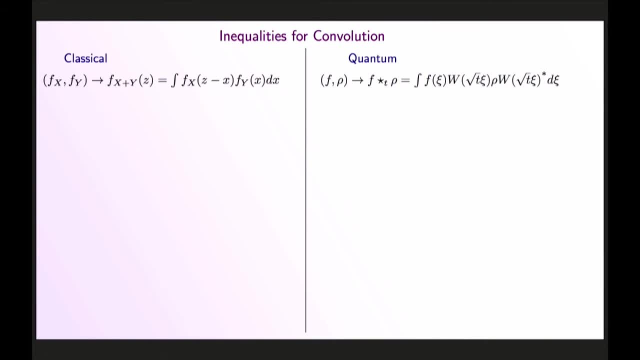 In quantum we use the one just defined. So the first one is Fisher information inequality. It relates the Fisher information of an added two random variables And the same one is the Fisher information of a convolution with the Fisher information of two independent entries. 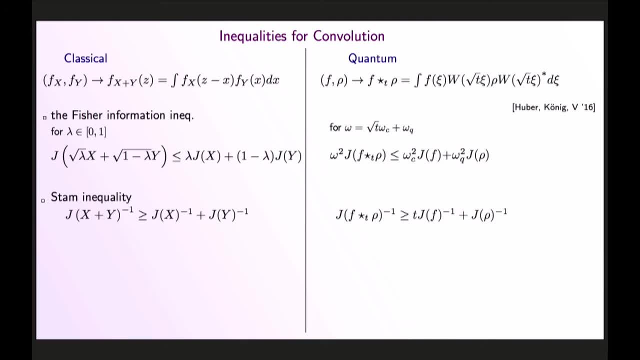 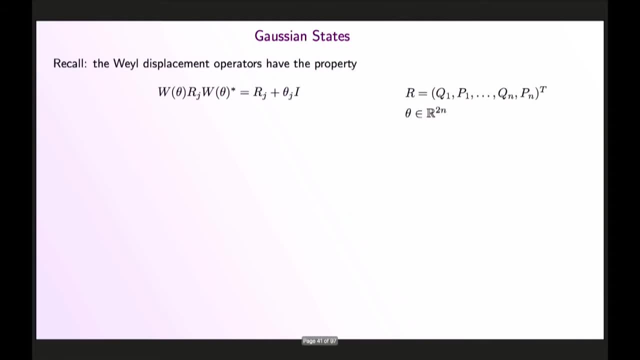 From here you can derive a stems inequality. It's just a simple one here and just an analog one in the quantum setting. Now let me first talk about Gaussian states. So just a recollection. We've seen them in two previous talks. 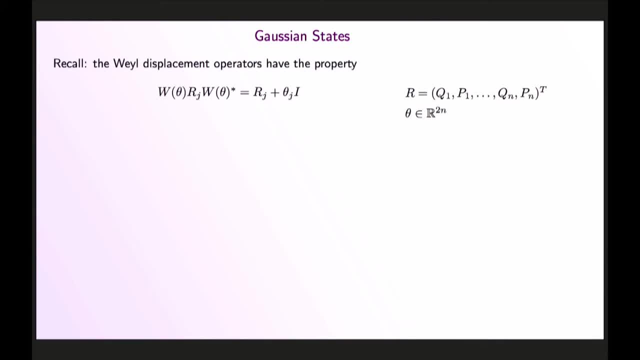 The Gaussian states are defined in the following way. So we have wild displacement operators that displace Q and P, And any state is defined by its characteristic function, which is trace of rho and the wild operator, or equivalently, by its Wigner function. 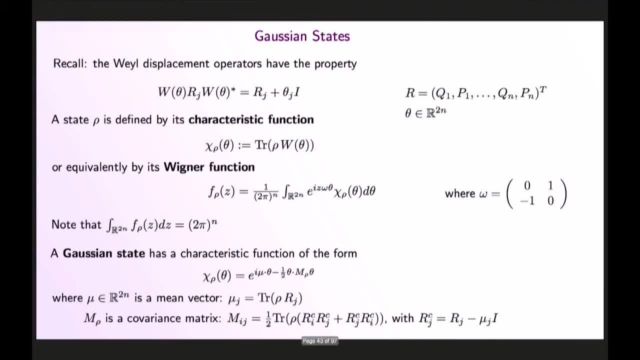 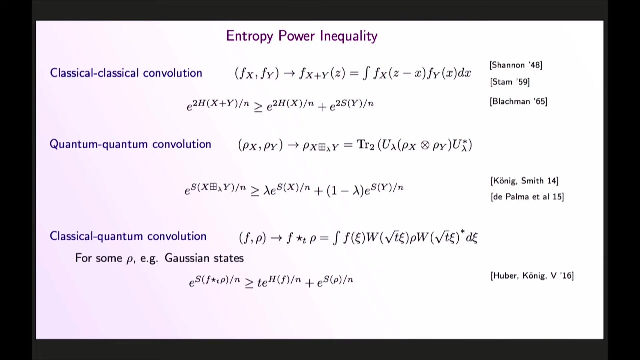 And the Gaussian states are defined by the characteristic function of this form. So we have mu, which is a mean vector, it's a trace, and m? rho is a covariance matrix defined like that. So for Gaussian states we can formulate the following: 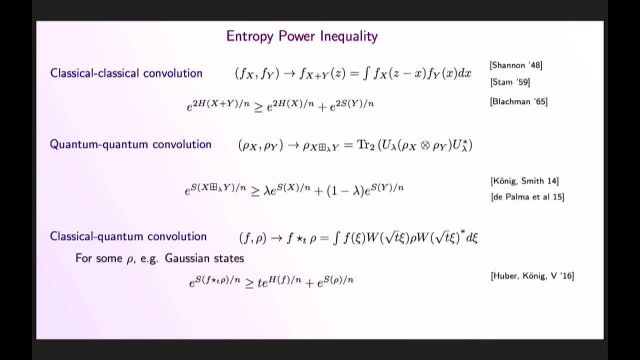 So entropy power inequality. For the classical convolution, the regular one, we have the entropy power inequality we've seen before. It was introduced by Shannon and then proved later by Stan Blackman in another paper. Then for the quantum-quantum convolution using beam splitter. 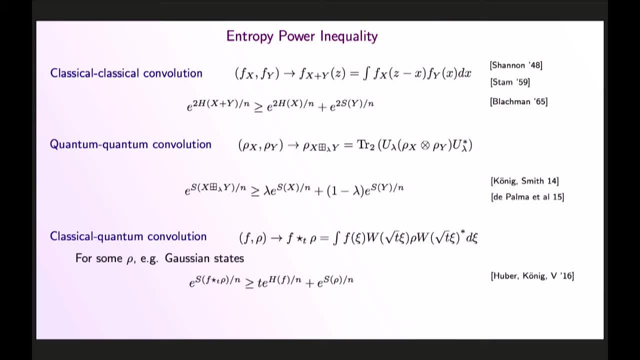 this was shown in 2014 and 2015,. Koenig and De Palma. And now, just to complete the whole picture, for the classical quantum convolution, we can also show the entropy power inequality for some states, in particular Gaussian states. 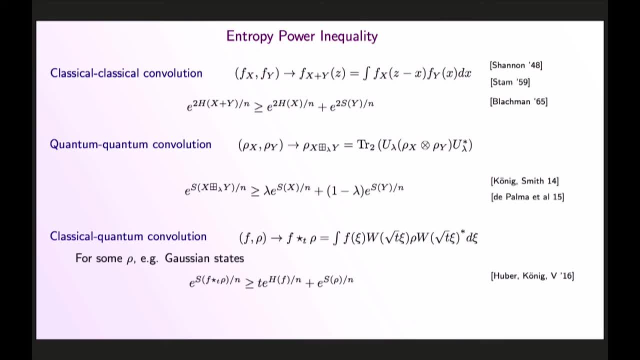 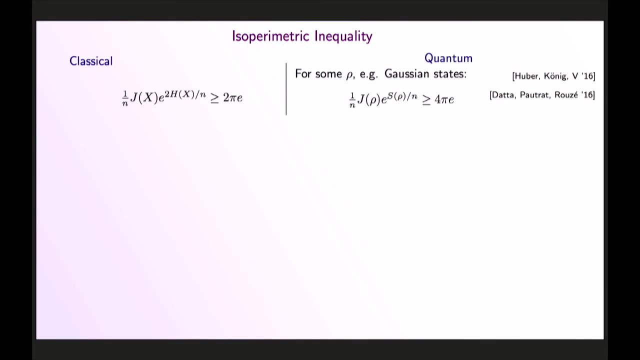 It's for a large class of states, but in particular Gaussian states. So the entropy power relates the entropy of the convoluted state with the entropy powers of two entries, classical and quantum one. Now for either parametric inequality. it's similar. 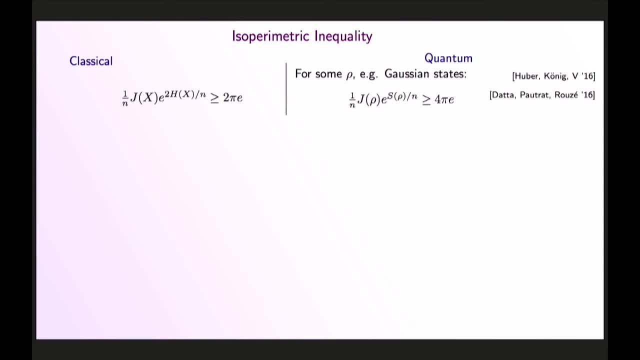 The classical one. we've seen before like that. And for the quantum again, for some large class of states, in particular Gaussian states, we can show the relation between the Fischer information and the entropy power. Now this inequality is tight in the sense that 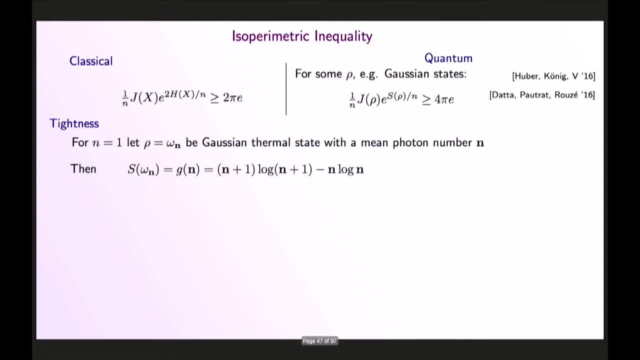 if we take a Gaussian thermal state, omega n, with mean photon number n, we can calculate directly what the entropy is, and under: Oh sorry, Sorry, that's not relevant. So by De Bruijn identity we can also calculate. 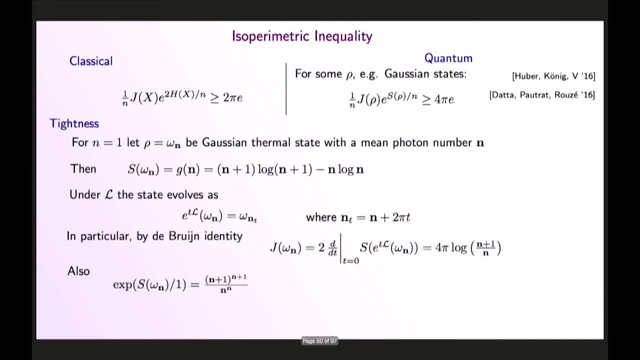 the Fischer information like that, And the entropy power is an expression of the mean photon number. So at the end we're going to have that. the Fischer information times entropy power converges to 4 pi e, which is exactly what we have here. 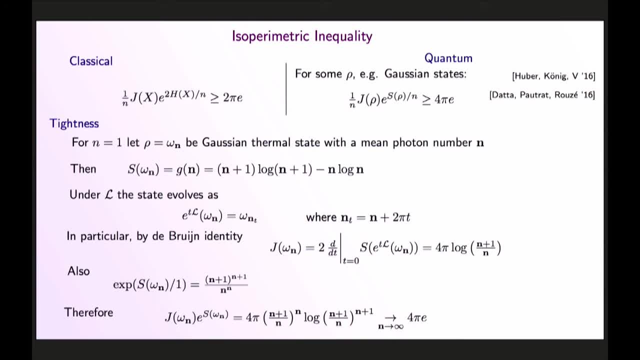 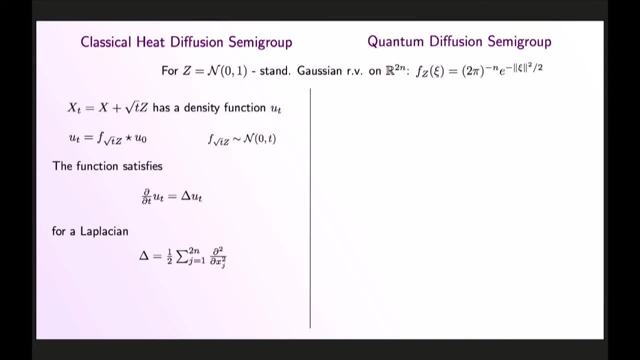 when this n is equal to 1. It's a one-mode state. Now let's talk about a diffusion semigroup For the quantum, For the classical diffusion semigroup. so if I take z to be a standard Gaussian random variable, 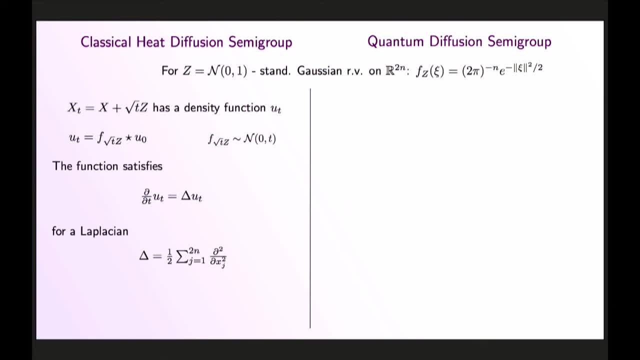 then The usual convolution is going to satisfy the differential equation where delta laplacian is a regular laplacian But similar in our case. if I take a Gaussian random variable instead of any function here, F, I can rescale it and my new state rho of t. 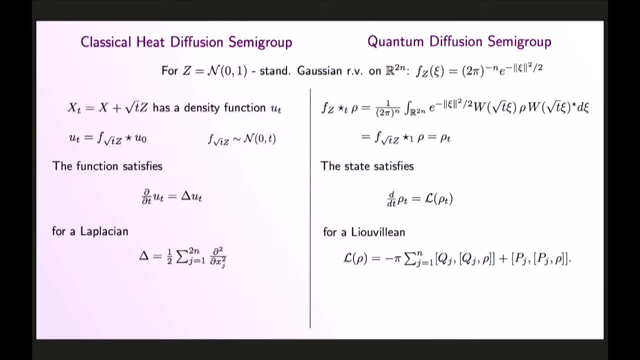 is going to satisfy the following master equation with L leuvelian given in this form. So this shows the analog between the new The leuvelian that I just defined with the laplacian, and that's why we call it quantum diffusion semigroup. 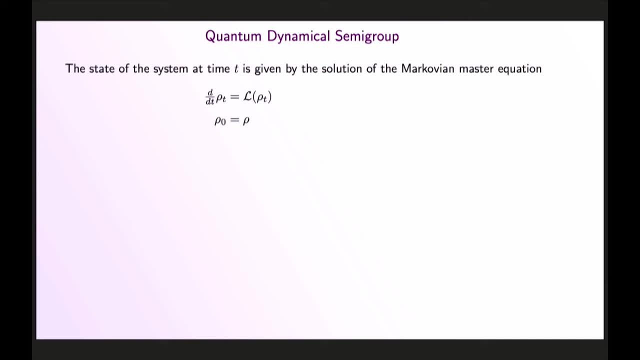 Now for this quantum. This diffusion semigroup generates a quantum dynamical semigroup with the regular properties of a semigroup lambda. It's completely positive, It's trace-preserving, It's identity on identity. It's a semigroup actually. 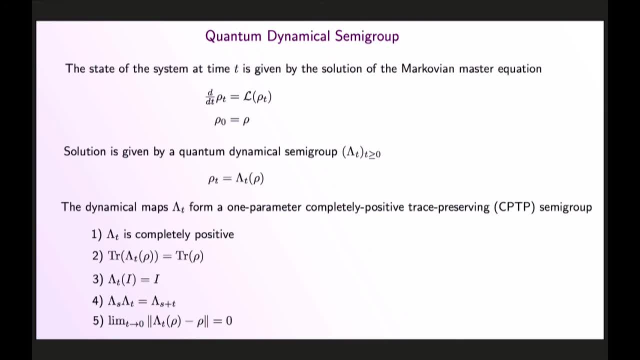 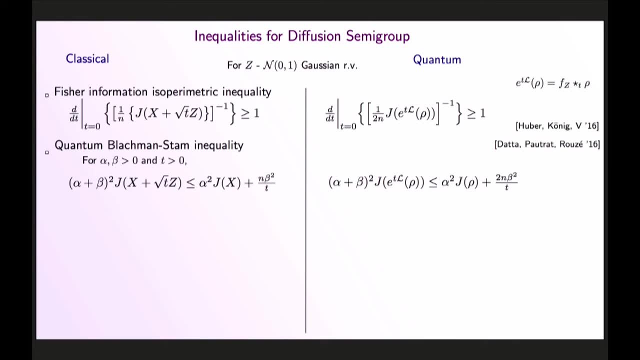 And it's completely, It's strongly continuous. Now for this diffusion semigroup, there are other inequalities: For the classical one, with the Fischer information as a parametric inequality, it corresponds to the classical one, So it's a derivative of the inverse function. 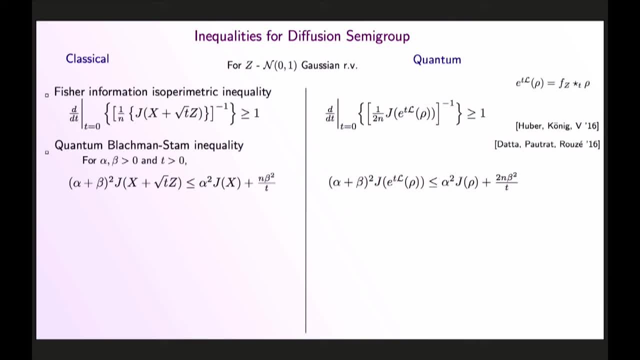 And from here the quantum Blackman stem. inequality follows, which relates the Fischer information of a time-evolved state with the original Fischer information, Now also for some class of states, for the same class of states I was talking about. 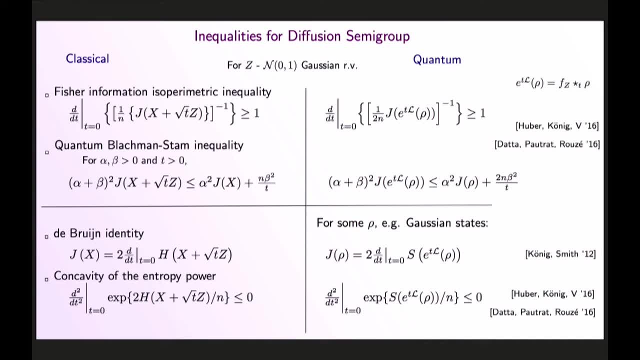 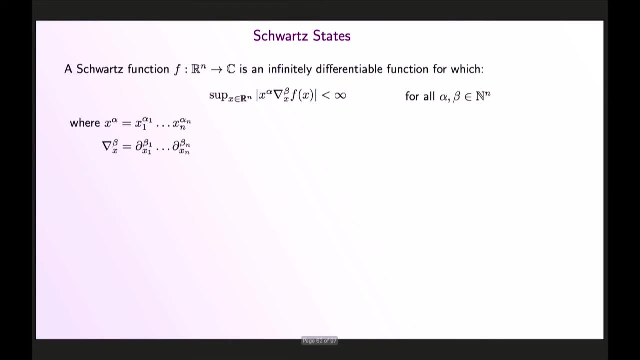 in particular Gaussian states. they bring identity holds, which was shown by Konig and Smith in 12.. But the new results are that also the entropy power is concave, just like in a classical setting. Okay, now also let's define Schwartz. 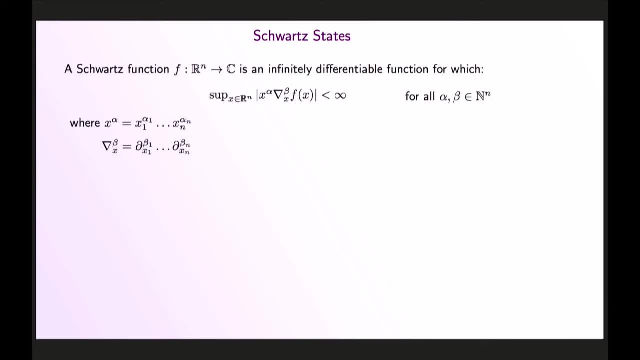 so the Schwartz function is Function F is infinitely differentiable function for which this supremum is finite and this gradient is just these vectors. So probability density function of a Gaussian random variable is a Schwartz state and the Schwartz state whose characteristic function is this: xi. 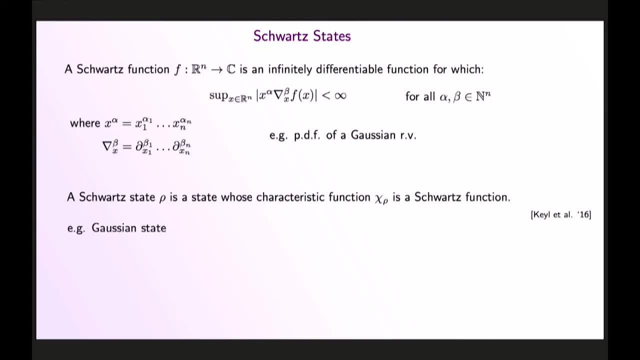 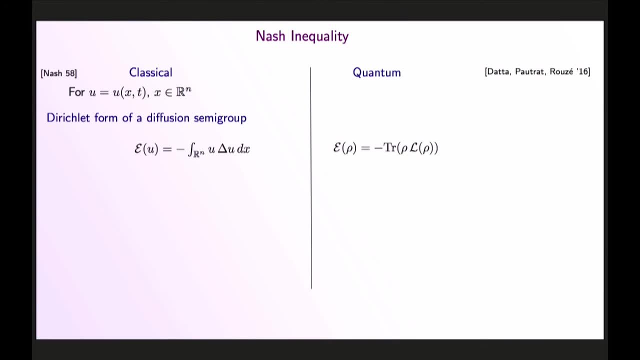 is a Schwartz function. So, for example, Gaussian states are fine. So for those states, for the Schwartz states, we can also prove the Nash inequality. So for the classical function u, let's define the Dirichlet form in the following way: 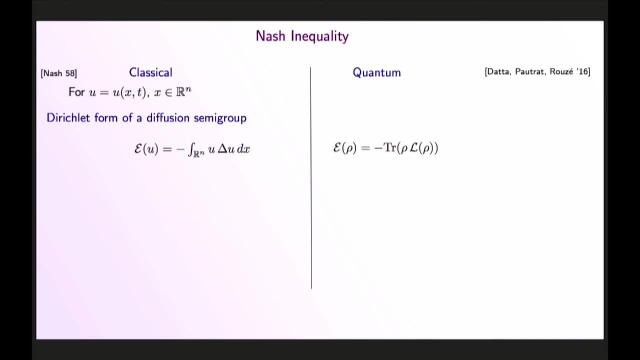 and in the quantum it corresponds, the trace of rho with l of rho And the Nash inequality then shows that there exists a coefficient that relates the norms of my function to norm, with one norm and the Dirichlet form In the quantum setting the Nash inequality is this: two norm? 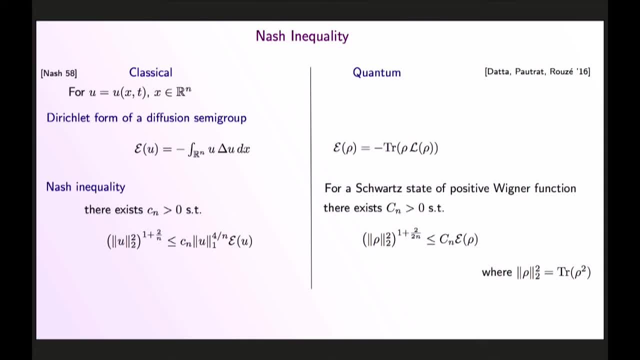 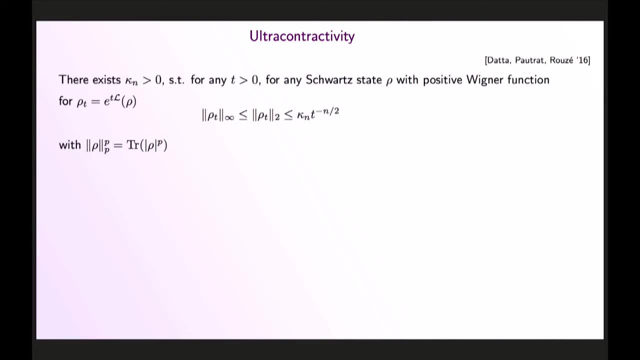 which is a purity of a state, how it relates to the Dirichlet form. Now for the diffusion semigroup. we can also show the ultracontractivity property, which means that for any Schwartz state with positive Wigner, function for a time of all states. 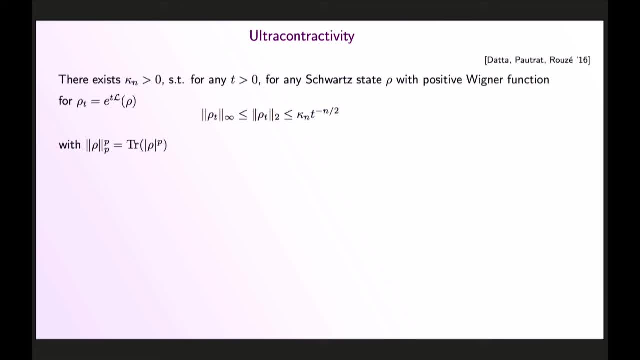 so the time of all states has a positive Wigner function and the original one is a Schwartz state, then the norms satisfy the following equation: So it's inverse power law decaying. So from here we can say that the purity has an inverse power law decay. 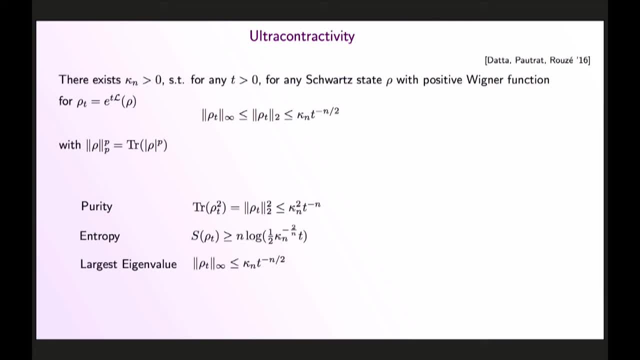 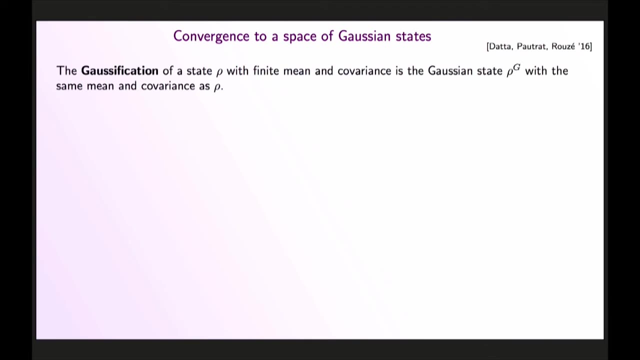 The entropy power has the following scaling, which is a logarithmic scaling, and the largest eigenvalue also has a power law, inverse power law, decay. Now the gaussification of a state with a finite mean and covariance is the Gaussian state with the same mean and covariance as rho. 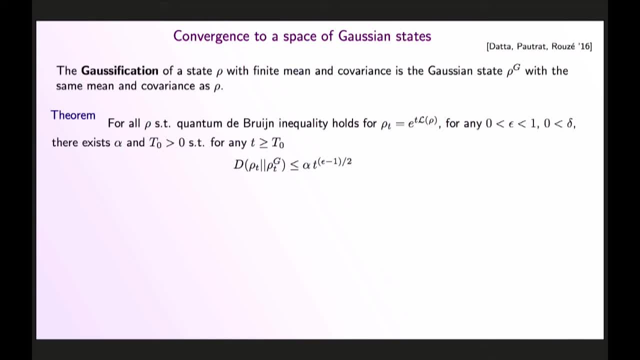 Now for all states, for example Gaussian states, for which quantum debris holds for the state, for the time of all states, there exist all these coefficients and times for which we show that the original state converges to the Gaussian state, to its gaussification. 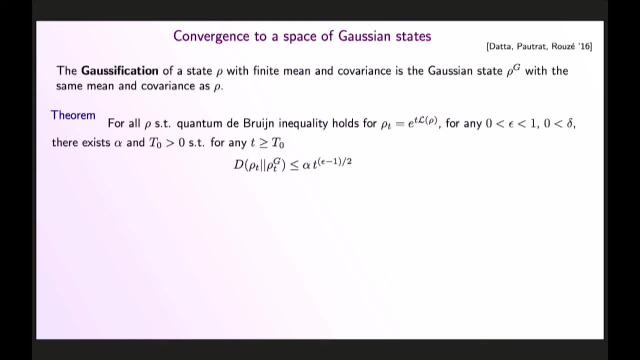 with power law decay And relating the relative entropy with the trace one norm, we can show that the difference of norms also has a power law decay. So classically it has the same property that, for a smooth function, the norm of the difference. 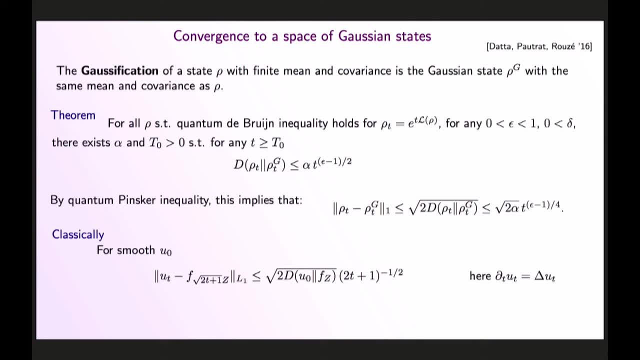 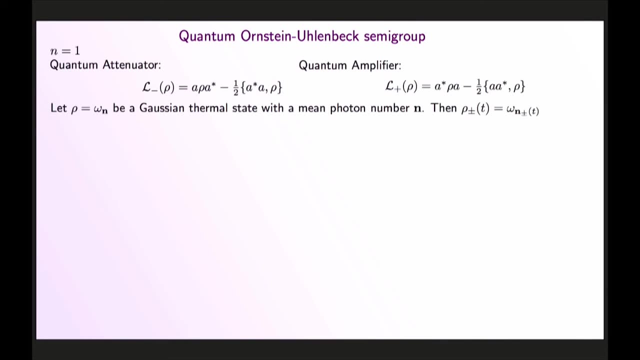 between the time of all function and the Gaussian function is related to the relative entropy between these two functions, the classical relative entropy with a power law inverse. power law decay here. Okay, now we can apply it to a quantum Orrstein-Ullebeck semigroup. 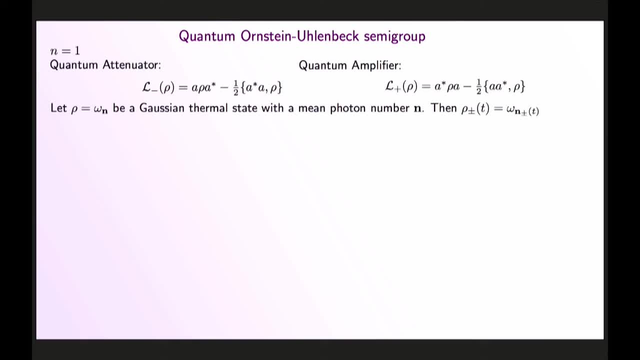 which is sum of quantum attenuator and amplifier semigroups. So if you look differently, separately, at an attenuator semigroup and an amplifier semigroup for a Gaussian state with mean photon number n, what we see is for the attenuator. 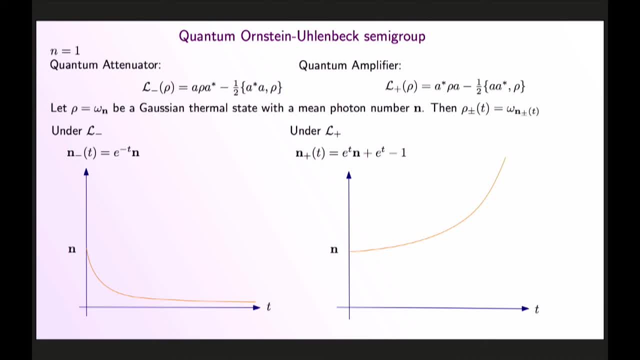 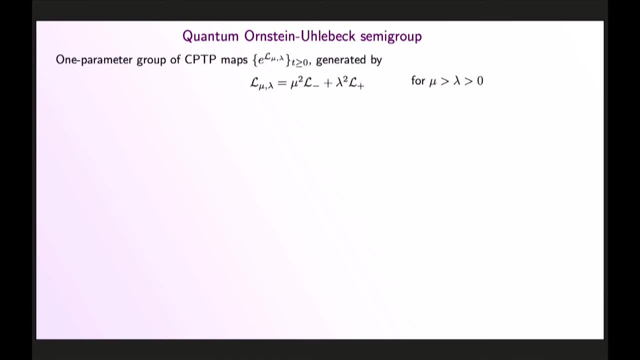 the photon number is going to decay with time. for the amplifier it's going to increase exponentially in time. So for the quantum Orrstein-Ullebeck semigroup with coefficients, let's say with coefficients mu and lambda, the mean photon number stabilizes in time. 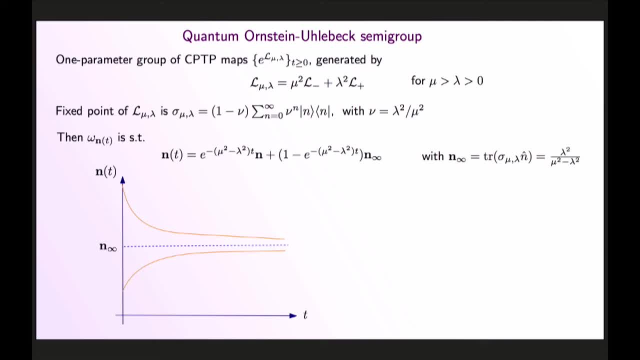 So wherever we're going to start, if we start here, it's going to stabilize to a fixed point of this semigroup, or if we start here, it's also going to stabilize Now we can show that for a large cost of state. 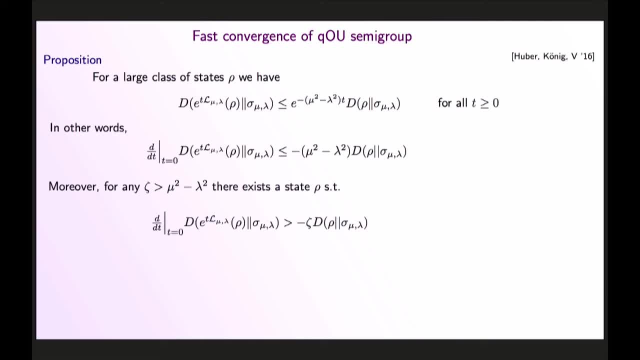 with, for example, small mean photon number or large entropy, we have that, the relative entropy of my state, time-evolved state. so my state is going to converge in time to the fixed state exponentially fast And this coefficient, mu squared, minus lambda squared. 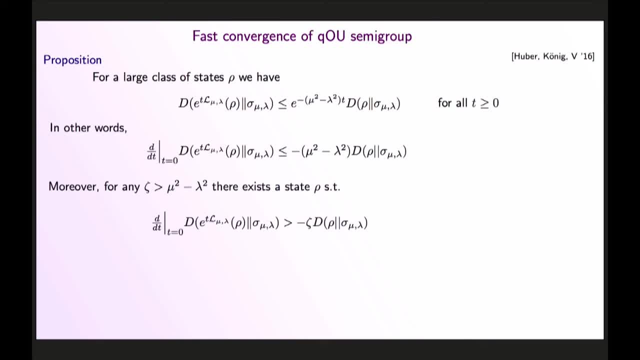 is optimal, in a sense that for any larger number there exists a state for which the inequality saturates, for which inequality is not right, And the conjecture was in June, made in June, that it's true for any state, not for just large cost of state. 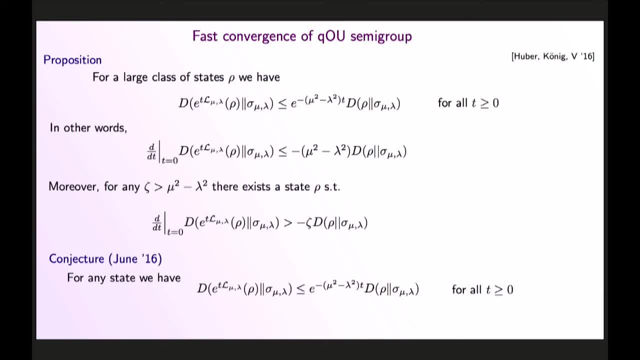 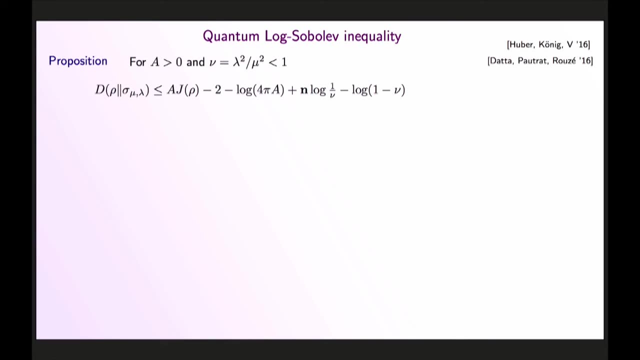 but for any state, our state is going to converge to a fixed point, and the conjecture was proved a couple months later using completely different methods. So just one last, just one last application to the quantum log-Sobolov inequality. 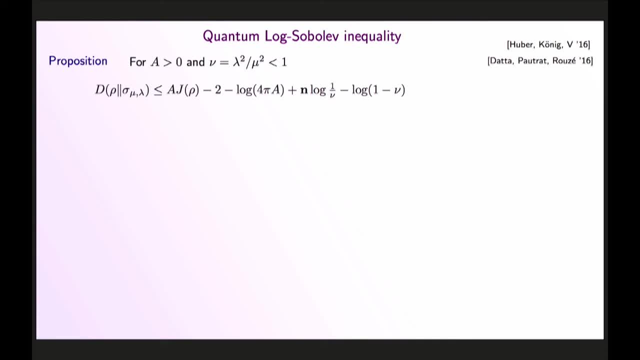 So that's, that's what I call the quantum log-Sobolov inequality. Now first, why that is true? because from isoparametric inequality we can relate the entropy and the Fisher information, the log of a Fisher information. 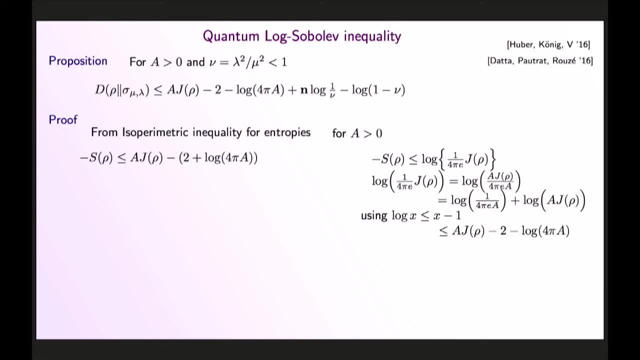 Taking log of this part and multiplying and deleting by A, we can write it as a sum. Using the next inequality: we can relate the log of the Fisher information with the Fisher information itself. So we ended up with this inequality From this inequality. 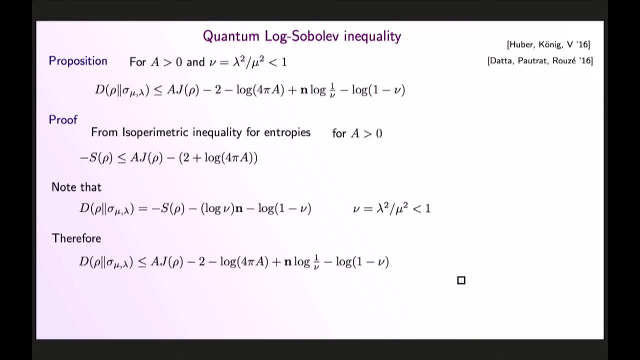 it's full, straightforward follows that the relative entropy. you can calculate it for for this fixed state, sigma the bit like that, and substituting this inequality for for the entropy, we ended up with the inequality that I promised. Now why do we call it? 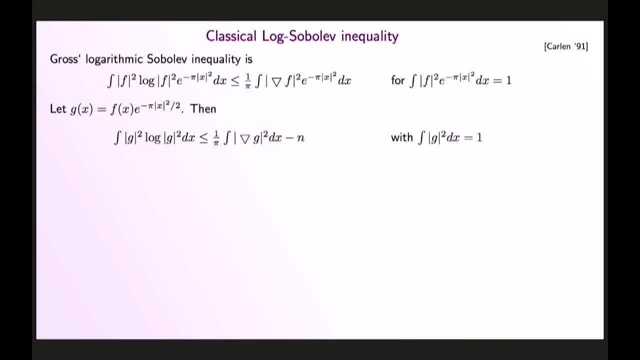 quantum log-Sobolov inequality. And this is the reason. The reason is the classical log-Sobolov inequality. So let's look at the classical one. So the classical log-Sobolov inequality is the following one: 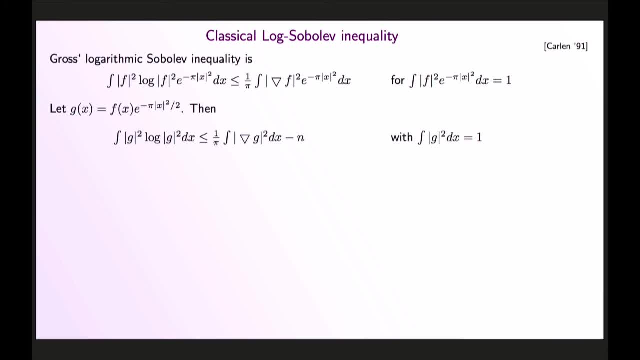 If here- so here is my function- satisfy this normalization condition. So if I take this whole function to be my new function G and rewrite this whole log-Sobolov inequality, this is what I gonna end up with. And now, 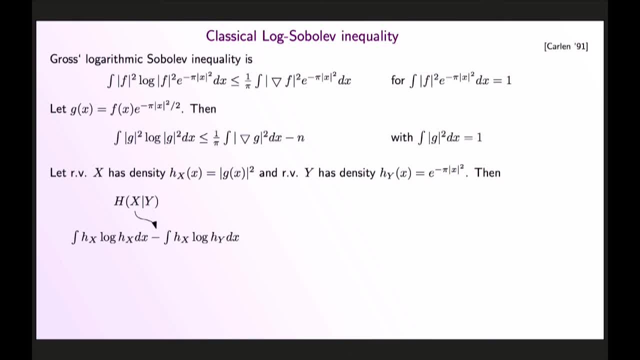 if I take a random variable with density function to be G squared and random variable Y with this exponential as a density function, then the relative entropy is gonna be this difference And the relative entropy. so this part, this part is exactly that one. 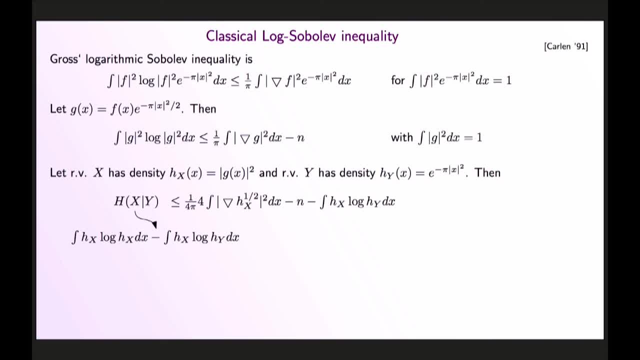 So I'm just writing it out Again, the inequality here and subtracting that part. But then you see, the first part is exactly the Fisher information And the last part is the second moments. So the log-Sobolov inequality. 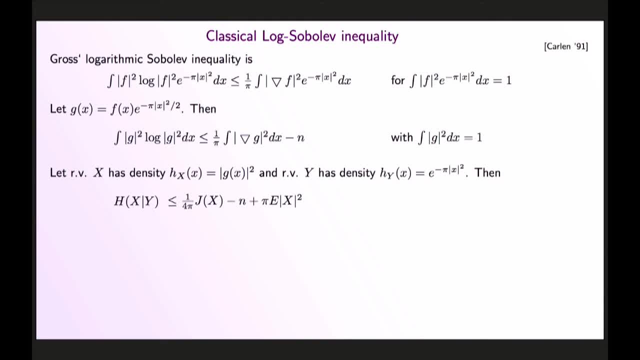 for the classical setting in the information theory looks like this. And what did we have for quantum one? We also had the relative entropy, the Fisher information and the second moments over here, which are N. N is the mean photon number, Then just some coefficients here. 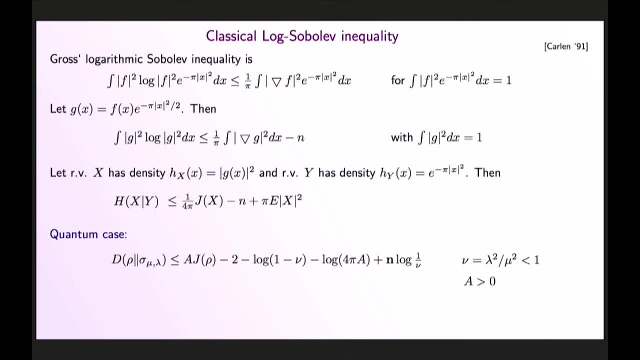 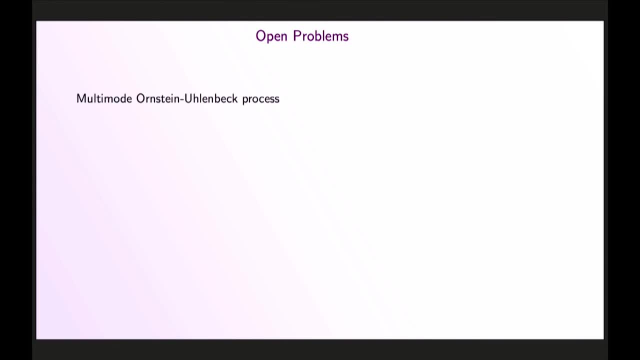 So that's why they're similar, And I'm gonna be concluding with open problems in a few minutes. One of the- the first one- would be the multimode process, because we had it only for one mode. Another one would be: 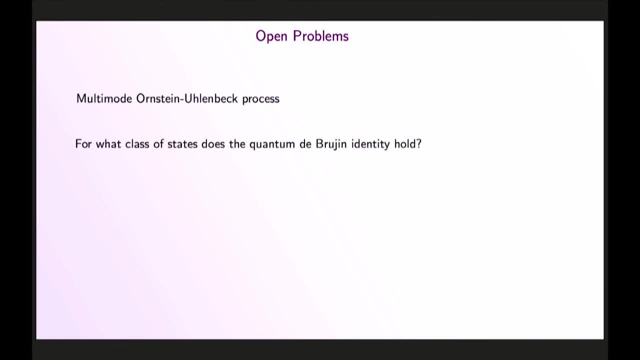 I was talking about the large class of states for which some inequalities satisfy, in particular De Bruijn's inequality. I said it's satisfied for large class, including Gaussian states, But for which class of states particularly it satisfies is still unknown. 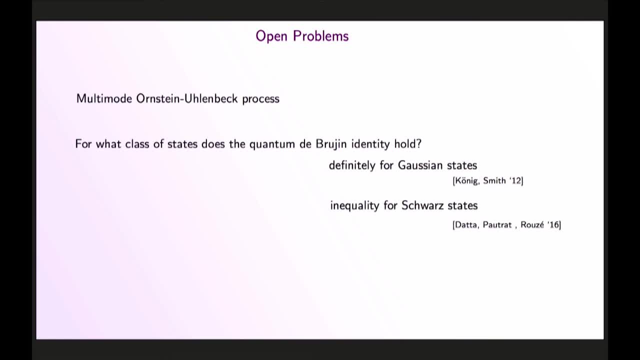 So we know it's for Gaussian states and data and others prove that it holds as an inequality for Schwarz states. But they hope it's gonna be equality for Schwarz states too, and maybe for a larger class of states. And then we also took 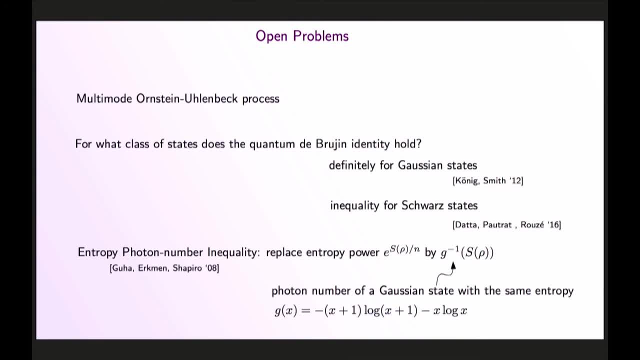 an entropy power as an analog of the volume. Remember, in the first part I was explaining why we took the entropy power. but instead of the entropy power we could take a photon number of a Gaussian state with the same entropy. That's also a good candidate. 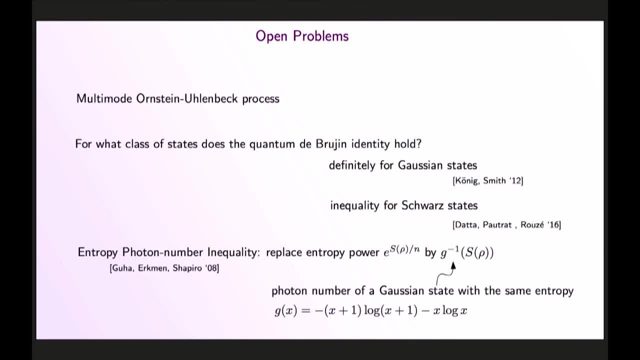 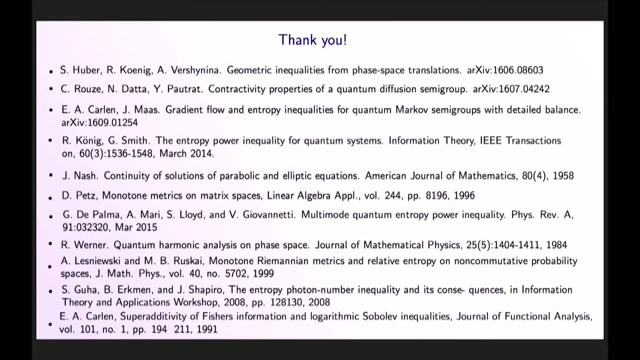 and if we do that, can we show any inequalities? Can we prove entropy power inequalities for this generalization? And that's this substitution was proposed in 2008.. Okay, Thank you. All right, Thank you. Any questions? I have one kind. 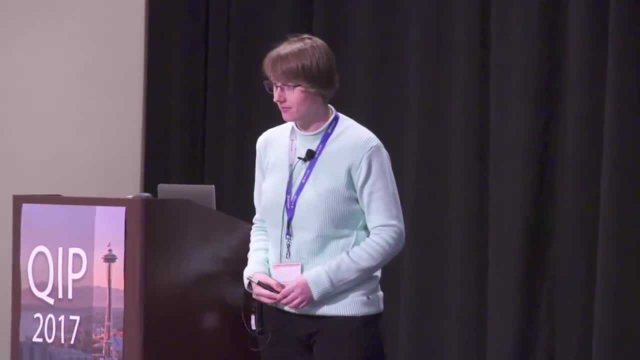 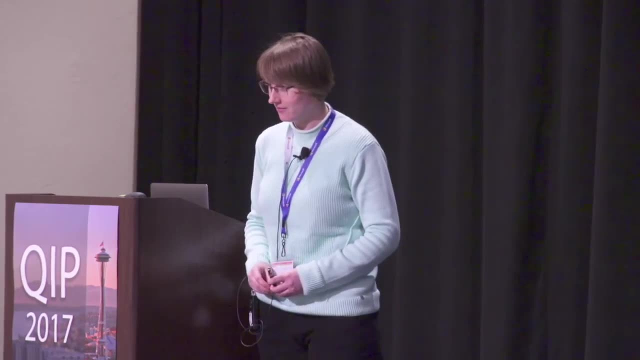 of general question because I'm kind of not very familiar with this field, but just read at some point that there are some physics applications where actually people you know consider this photonic equations and some control experiments. So can you comment on this? 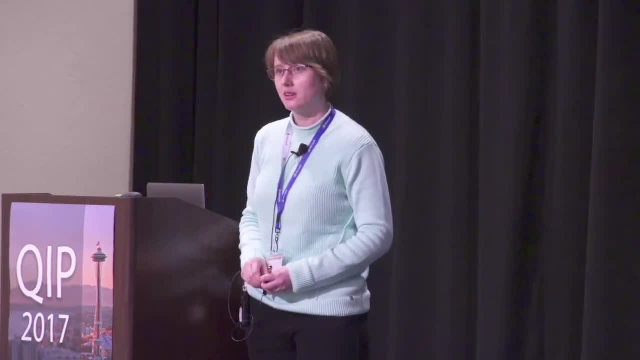 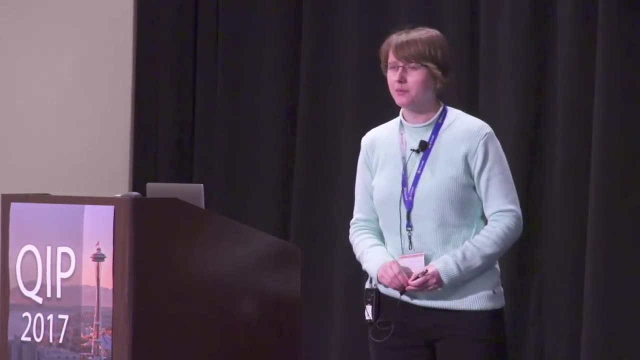 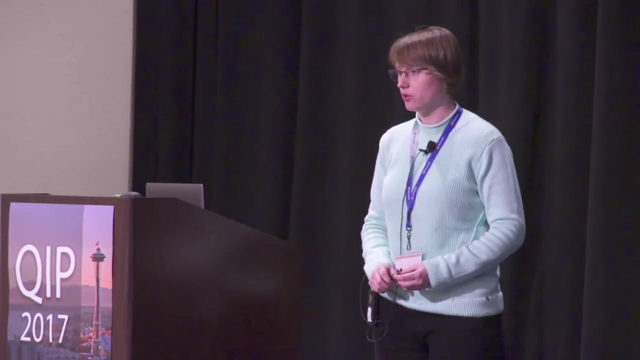 Are there any experiments that do this stuff? Or you know where it's used for control or something like that? Right, Well, I'm not aware of any experiments, but these inequalities, they're used to bound the running time of algorithms. 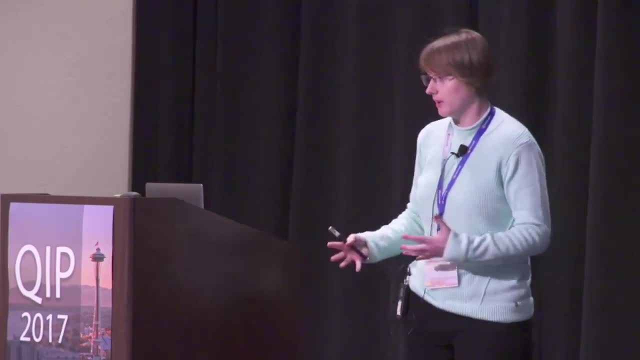 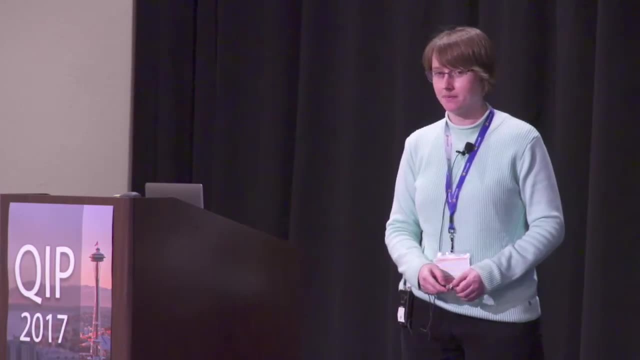 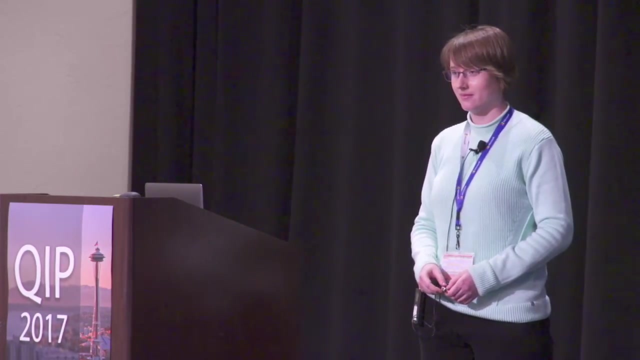 so it's not exactly experimental stuff, but it is relevant for experimentalists. Any other questions? Okay, Well, if not, let's thank all our speakers from this session again. All right, Thank you.